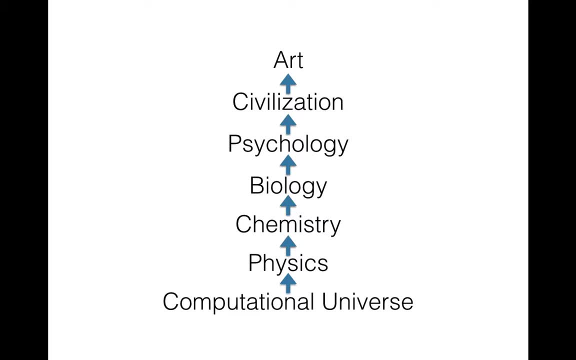 So we were here, right, Are you with me? Yes, you are. Now, when do we start getting really mesmerized by the stuff that we see is the level of biology? Okay, Do you agree? Okay, Like something, like standing up and walking, It's really, really something. a. 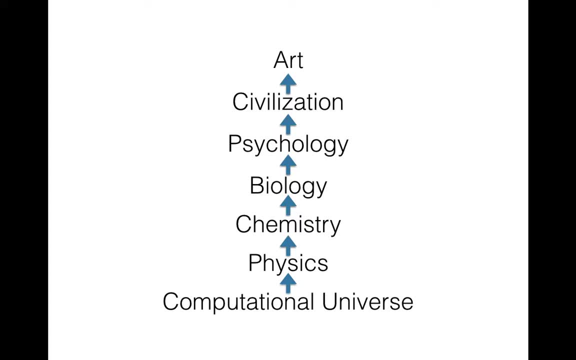 joy forever. right Now, I will again speculate that it comes because of this loop backwards loop. It's not just a feedback loop. We have feedback loops downstairs as well. It's a strange loop. to borrow Douglas Hofstadter's words, It's a strange loop and the strangeness of this loop will. 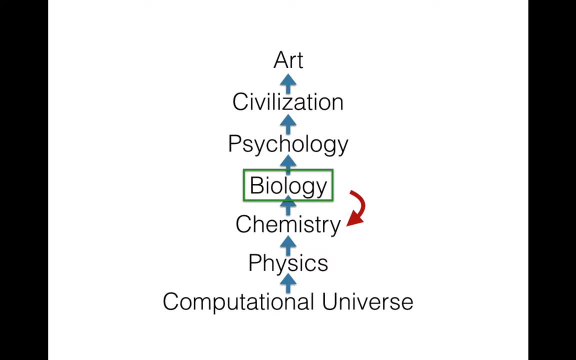 be apparent, maybe in a couple of minutes, or maybe never. But the strangeness goes to the upper layers as well. Our psychology may influence. Well, basically, biology has this freedom of changing its rules. It's a very important freedom- changing how it is built. That also makes it computer science. 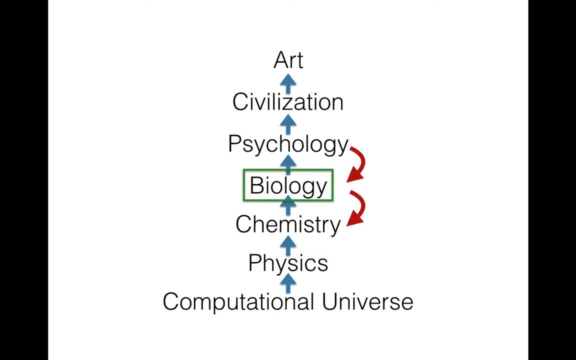 right. Think of a program that can change its program. The possibilities are infinite, right. And then civilization can affect your psychology while being an emergent property of the sum of your psychologies. Okay, Do you understand the dynamics here? You make the culture that you are living in, but 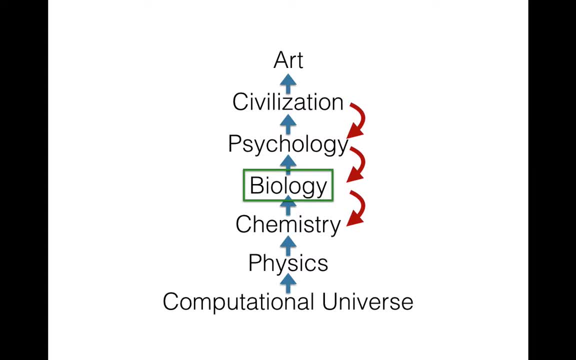 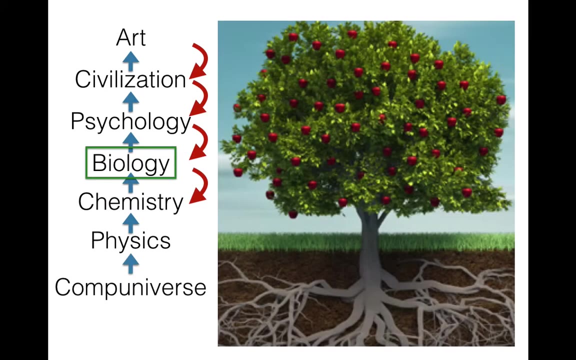 you are also affected by the culture that you are producing backwards. Does it make sense? And art comes back and affects civilization as well. So in a way, we can imagine a tree that is no longer human but that is going to be in the future. 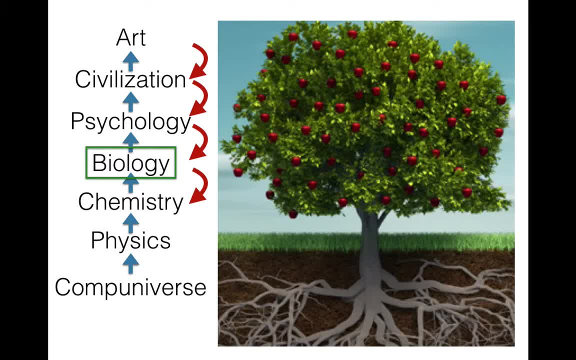 Okay. So what we have to do is to create a new world that will be a new dimension, Okay, And I think that the world of the future. we have to create a new dimension and we have to create a new universe, Okay. 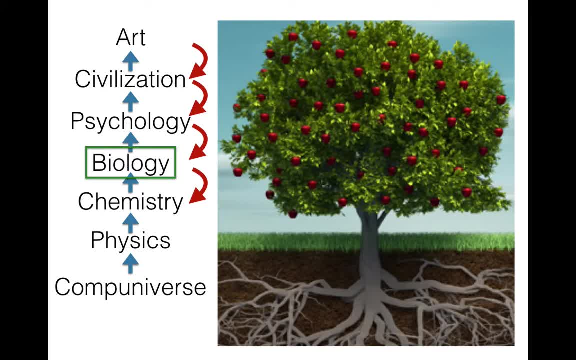 And so we have to start to think about what we call a four-dimensional world. Right, And when we think about a four-dimensional world, we think about the future of our universe. Yes, exactly So we have to think about the future of our universe. 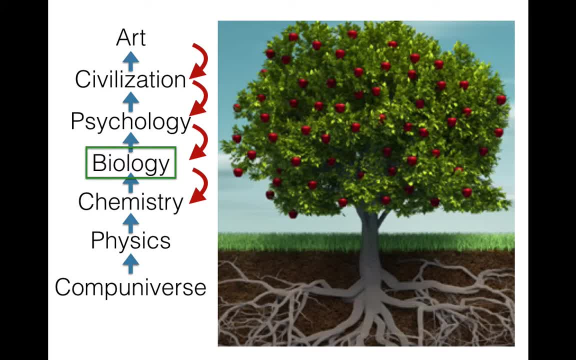 Right, And we can only see it mathematically. We can understand it, But we haven't been evolved in a four-dimensional world universe. That's why we cannot imagine a fourth dimension, right? Yes, that's the reason why people usually tend to go when you, when they go to. 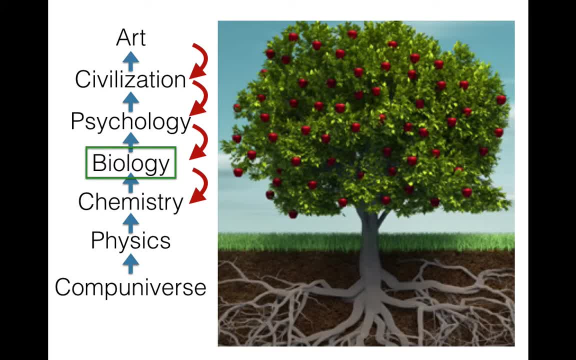 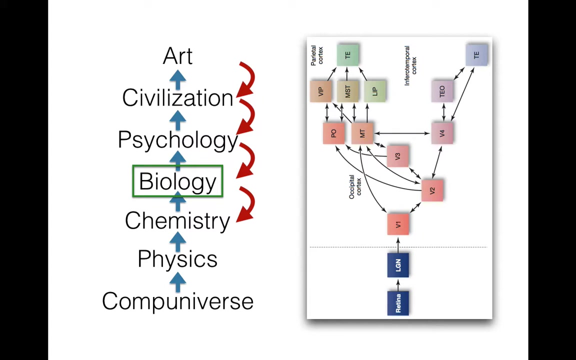 ultimate theory of reality. they use 11 dimension, 26 dimensions. there are good reasons for that, but you can imagine a tree, its roots that are not seen are downstairs somewhere, then there is this physics, then there are these branches, and all the beauty and the fruit is art. but yes, and okay, it was a joke in. 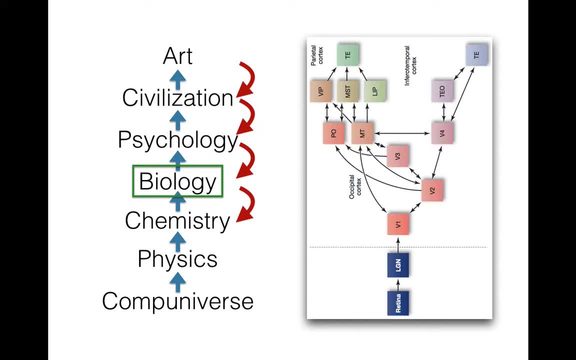 Turkish. sorry for that, and let's make this strange loop more apparent, like let's try to explain it by giving an example from your brain and how, in particular how you process visual information, you can see that there are a lot of things that are happening in the world. 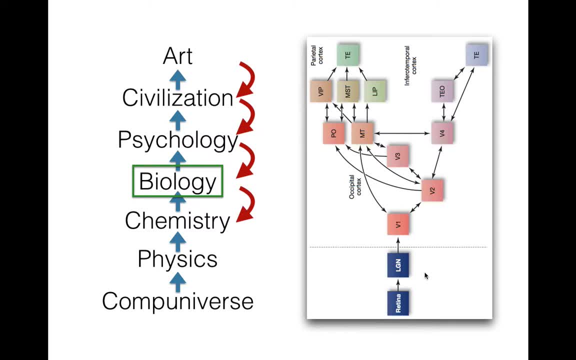 basically, it comes through your retina, goes to LGM. what is LGM? no, sorry why I didn't point at you at first: laterals geniculate nucleus. thank you very much. it's doing a linear process. it's doing something that it doesn't care what happened next. Okay, so it takes in the 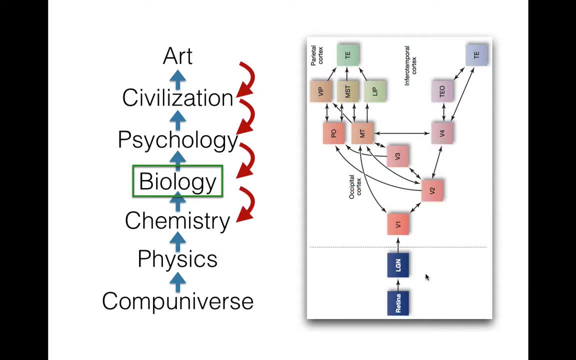 information. what happened there? Just like feed forward, neural networks takes in sense it up, doesn't care what happened, okay, But once it comes to V1, It does care. it gets affected from the information that was sent upwards because it goes Enters to this strange loop. We can see that it's not just one loop. 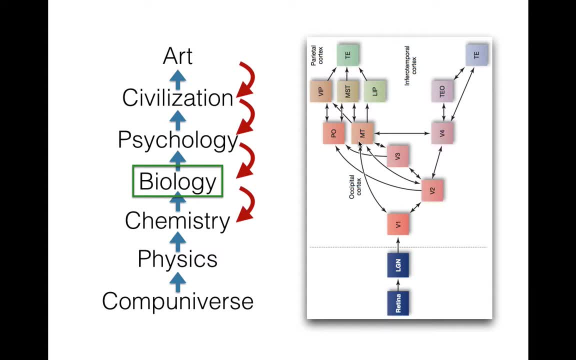 That's just. it's not like just Krebs cycle, Which is also a strange loop, because there are loose ends that are connected to other metabolic activities, right, It's the whole metabolic network. There you go, Another strange loop, right? so wherever you see richness, you should seek for a strange loop there, and 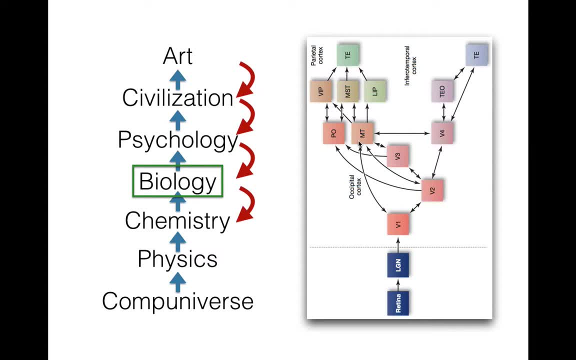 visual system, visual processing or consciousness, is Something very interesting, and it is a result of A strange loop. another speculation, Yes, But you should also read Douglas Hofstadter's I'm a strange loop, Okay, So let me show you how it works. I will show you five shapes. 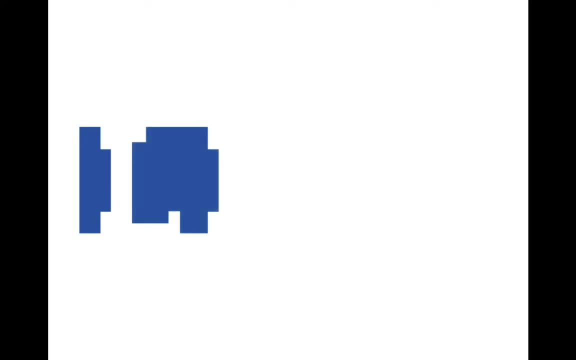 psychology test. okay, first shape, second shape, third shape, fourth and fifth. Does it make any sense to you, those who haven't seen this before? Have you seen it before? You are one of those rare people who look for The letters. when I told you to look for shapes. 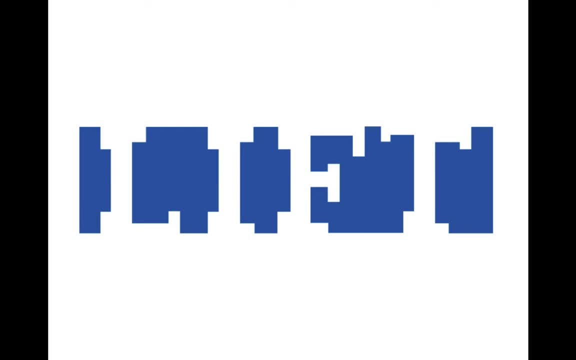 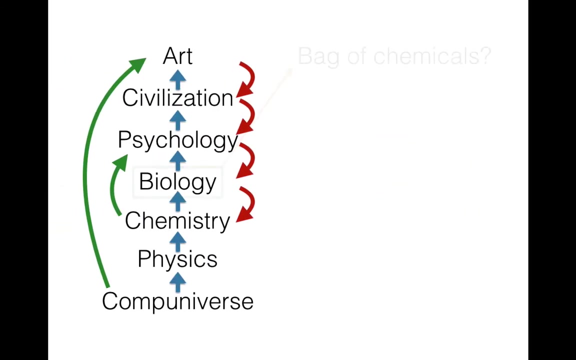 When you see the letters written in white, You will be unable to unsee them. but before you couldn't see them, right? Something changed in the upper loop and now you just cannot but see it. Do you understand the point? Yes, So. 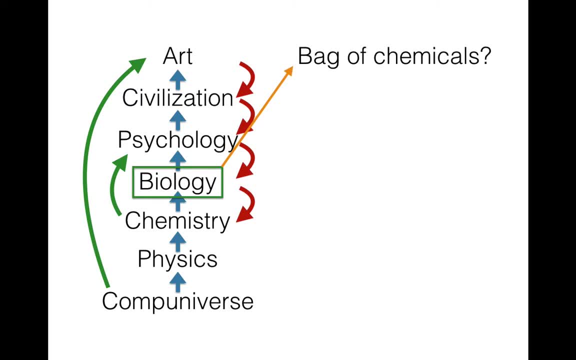 Are we bag of chemicals? Yes, of course. so if I take your chemical Stuff, put it in a bag, shake it, Will it make a nice Doran? There is something extra there, right? Well, my point is that no, we are not bag of chemicals. we are bags of chemicals. 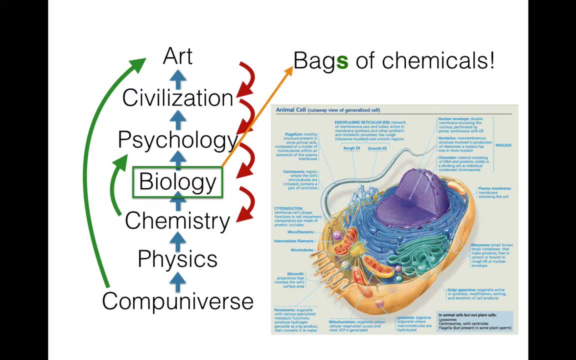 That's the difference. That's the difference because that's the way To build this strange loop, because you need levels of organizations that are made Possible by these bags of chemicals. just look at the cell, a unit of life, And you will see bags inside bags, inside bags inside bags, etc. 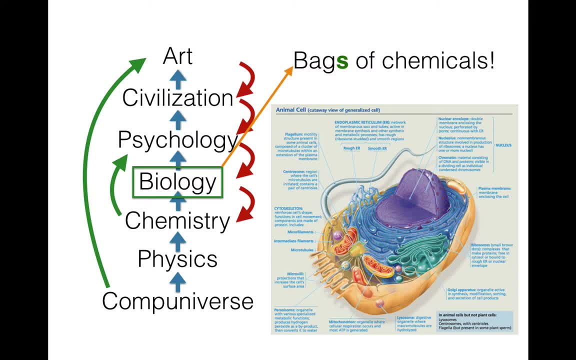 right, these bags, bag baggy organization makes possible things that are improbable, so like You need something to be broken down chemically, right, If you leave it outside, it won't be happening anytime soon because the pH is not enough. Okay, but you have this lysosome. if I'm wrong, correct me please. 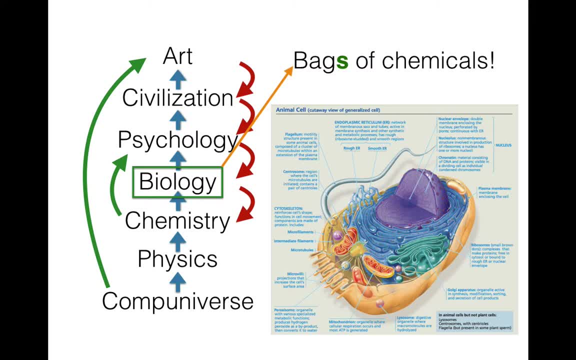 Yeah, you take in that stuff. It Ments, it comes together with the lysosome. that inside it has a lower pH- I believe much lower- which breaks it down for you. So you make something improbable possible because of the back of the lysosome, where you create a special specific structure. 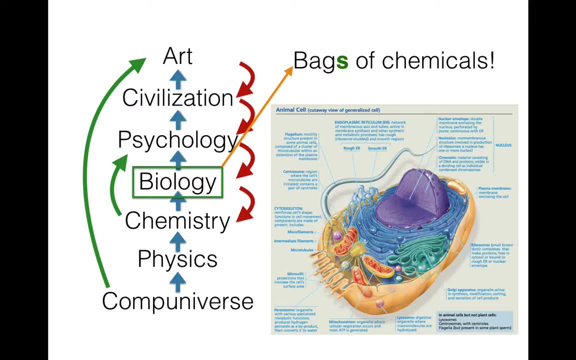 besides being low pH, it also Enables things to react much more because it's inside a small bag, So a possibility of banging into each other is much more, much higher. I Thought that it is an original idea, but Apparently there is a person who is Studying it and it's called- he's calling it- Markov blanket. Okay, these things and 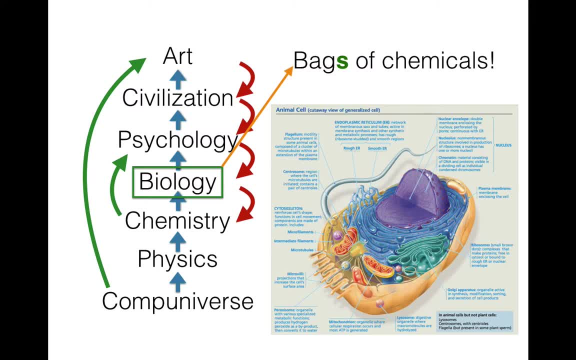 Those who are interested in it. you, you should search for it. You had a question. Do you use the same method of reproduction to go up to the level of the intracranial membrane? or biology? There should be at least a brain and few neurons to have a psychology. 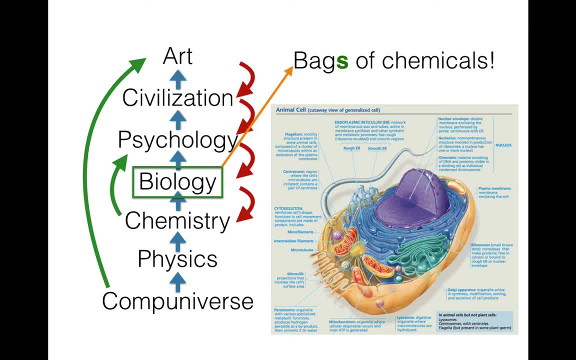 or from psychological civilization. there should be at least a few psychological entities to have a civilization. Yes, so the question is: do we need many actors of a certain level of Organization to build the upper level of organization? is that the question? Yes, right. do we need the upper level organization to build the upper level of organization? Is that the question? 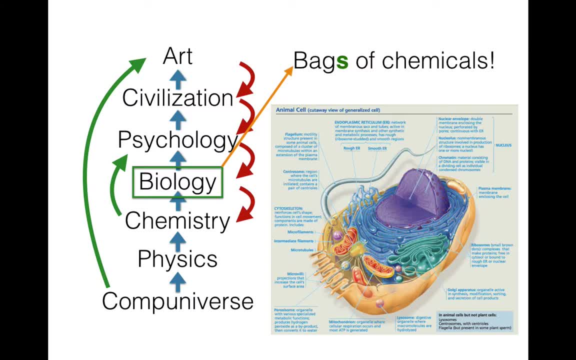 Okay, Do we need three entities? No, you need much more. You need like 10 to the 11,, 12 or whatever, 10 to the 23 to go from chemistry to biology. right, Like molecules by themselves have some interactions, 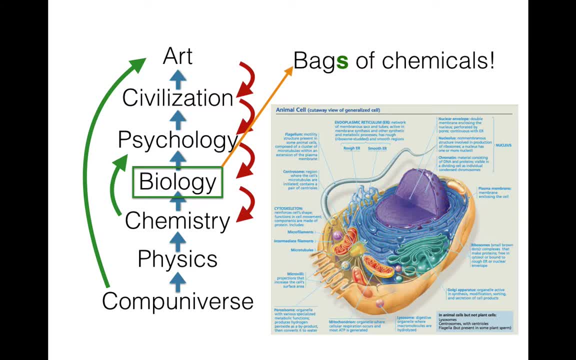 but the emergent properties that biology desperately needs, like pH. okay, For example, you use pH in biology right As just a number, But pH is an emergent property coming out of 10 to the 23 molecules of water. 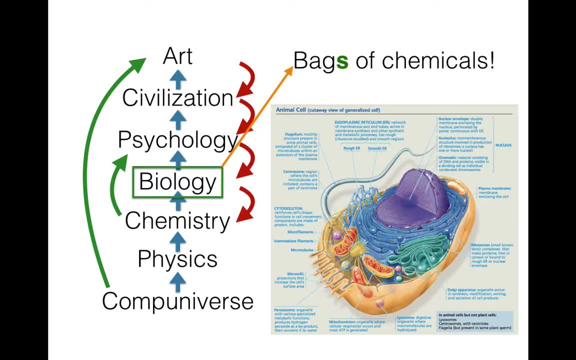 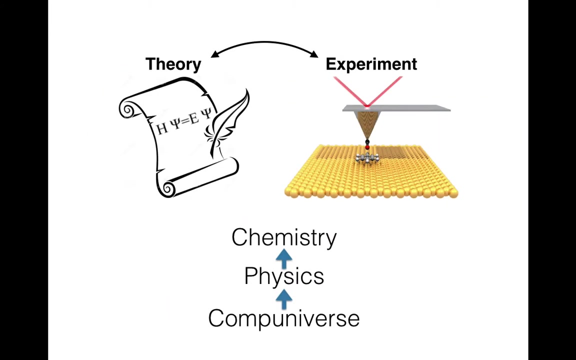 Some of them has extra hydrogen, some of them has missing hydrogen, which results in a global pH. Am I right Or wrong? You have to say something. You are the judges. Chemist, Yes, Yes, Okay, So actually we can skip this part, very, very quickly. 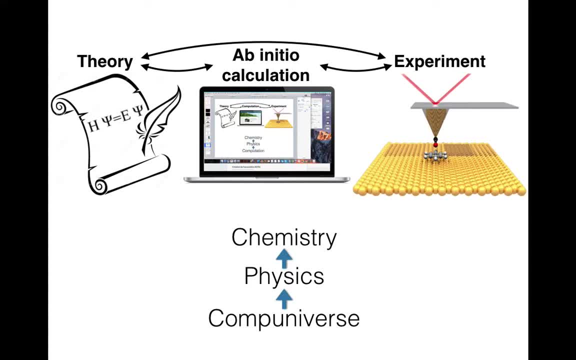 This is what I have been doing for 10 years. It's basically using this arrow. that is quite straight. So you can, just as I mentioned, if you can solve Schrodinger equation, you can talk about chemical properties or material properties. 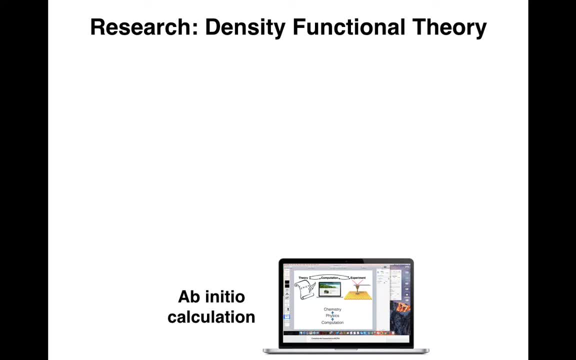 And the problem with solving Schrodinger equation is that I will not explain you why, but you can read it later on- If you want to store the wave function of nitrogen atom- it was a final question in the previous course- It works. 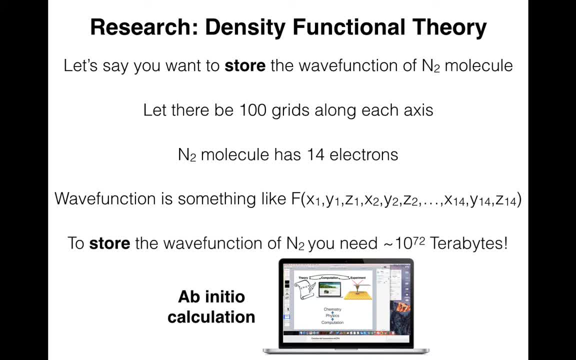 It was oxygen, but it doesn't matter. You need 10 to the 72 terabytes just to store the wave function, not to calculate anything, And it's even undoable. Do you agree with me as a physicist? Yes, Yes. 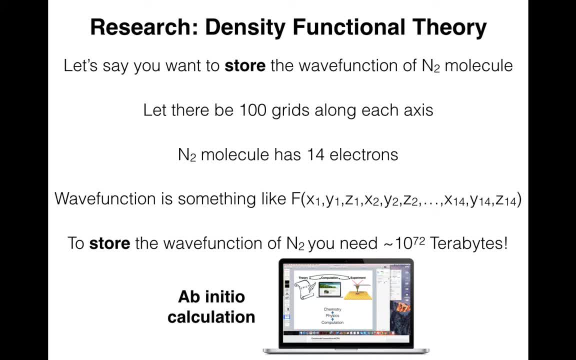 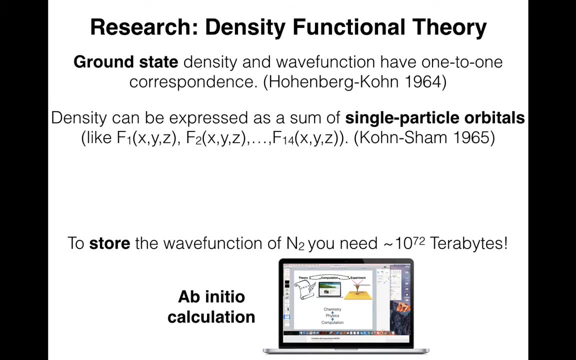 So you cannot solve it. You cannot store it. to solve it right, All particles, if they are hard disks, cannot. You cannot take up this information in. Well, what do you do? You use this nice theory, test functional theory. 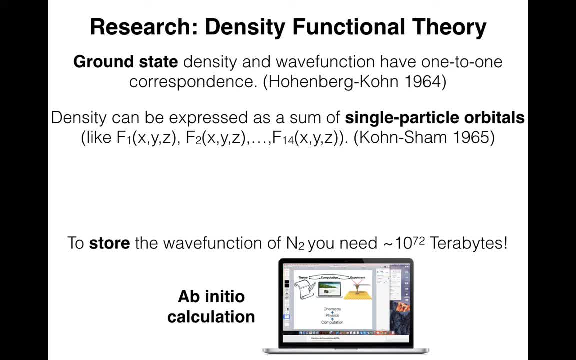 We use this theory to map this gigantic wave function into something that is dealable, And it works Okay. It shrinks down to 10 megabytes, sometimes even smaller, And you can make calculations that are precise enough, for It's a very simple prediction. 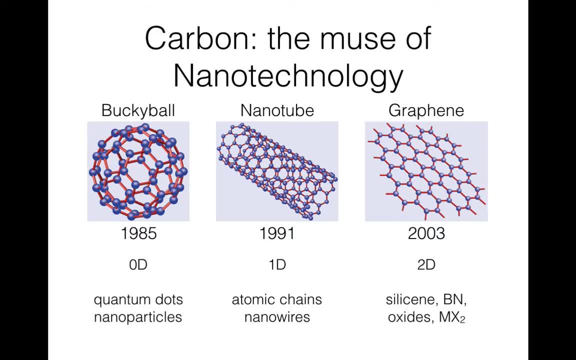 And what we did. this is just me talking about myself, So it's boring, I know, But carbon basically decided what is going to be next in the field of nanotechnology, It's allotropes, So the most popular one very recently is graphene, which opened the door for 2D materials. 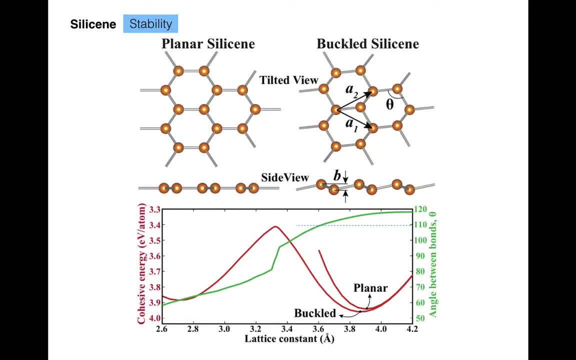 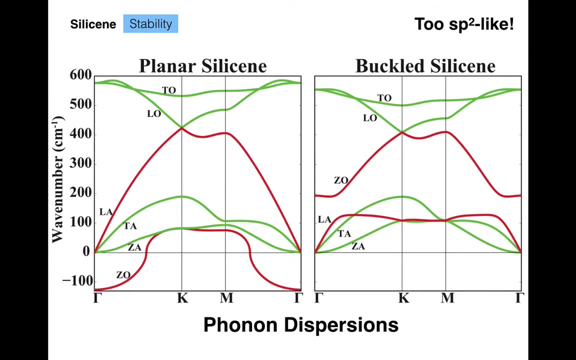 And what we thought was very simple: Why don't we replace carbon with silicon? Because we like silicon, right, It's in the devices, et cetera. We realized that it's not really stable in the graphene-like planner configuration, But it can be made stable with buckling. 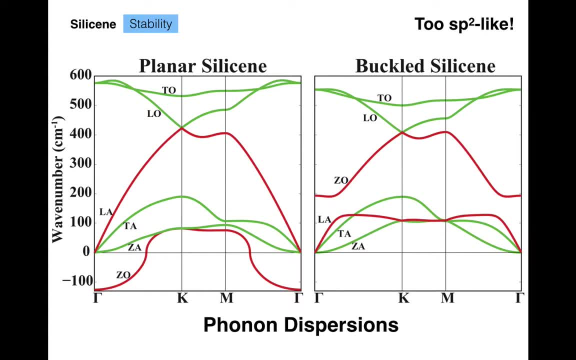 So let me remind you, we are doing all this in a computer. Okay, So this is an exploration in a computational universe. This is the search of a novel material that hasn't been synthesized or found in nature. Right Then, basically, this plot shows you that this material, if it is synthesized, will be stable. 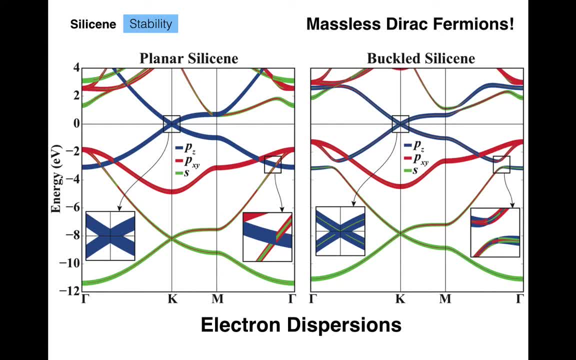 Right, I will not tell you why. And it will have this nice property of electrons acting as if they are light particles, So-called massless Dirac fermions. Do you realize that electron, normally that has a mass, particle that has a mass inside this material, it feels like or behaves as if it hasn't got a mass? 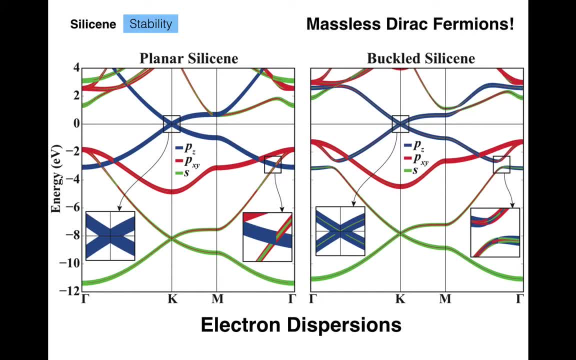 Right. So what you can derive from here, what we mentioned earlier: don't trust even the most physical quantities. They may change in different situations. Do you see the point? Even mass is an emergent property. Okay, So this is our paper. 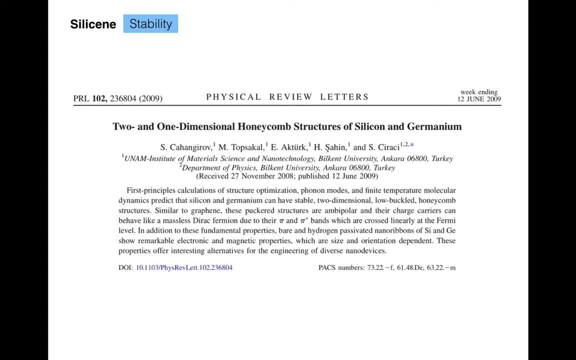 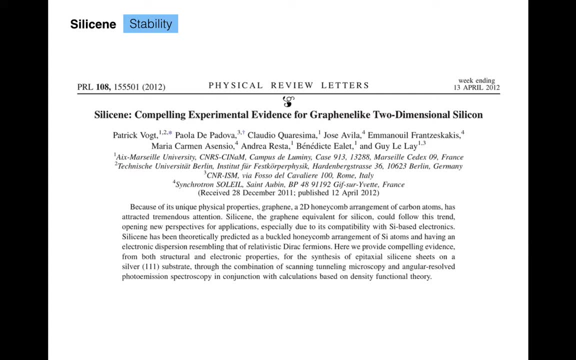 And it's in 2009, from this building, And this is after three years. it was synthesized- Yes, it was synthesized, not freestanding on a silver surface, But still it's out there, And it had a huge impact in the literature. 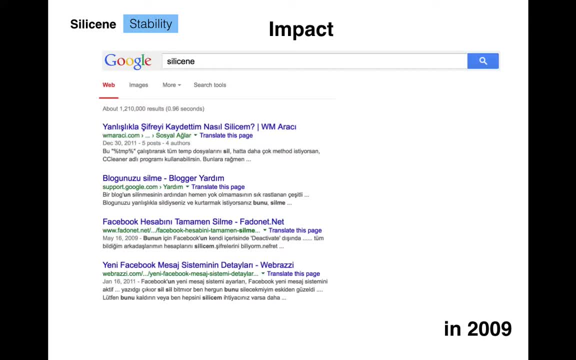 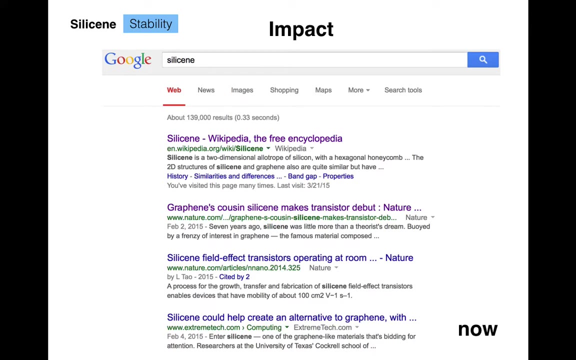 Back in 2009,. this is what you would get if you would Google it. Okay, This is what you would get if you would Google silicene. Instead of erasing that, erase this Now. if you Google it, you will find. 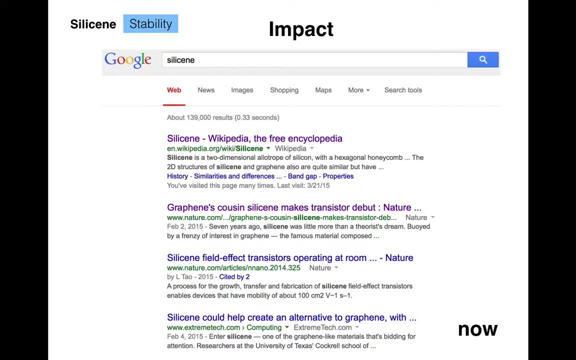 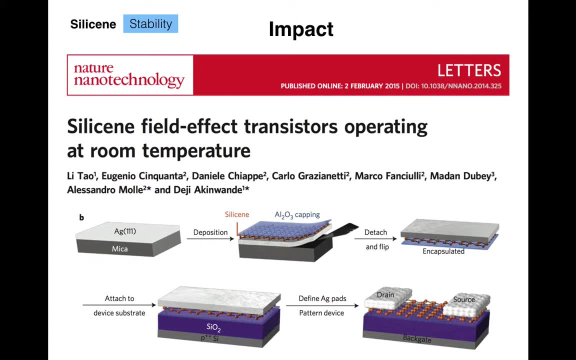 And all this started with an exploration in computational universe, Do you see my point? And people even made field effect transistors out of silicene, Although they operate only for 10 minutes. those are in smaller captions, Okay, But it's still. I mean something going forward. 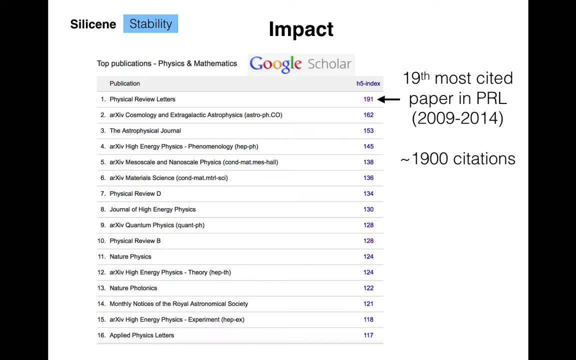 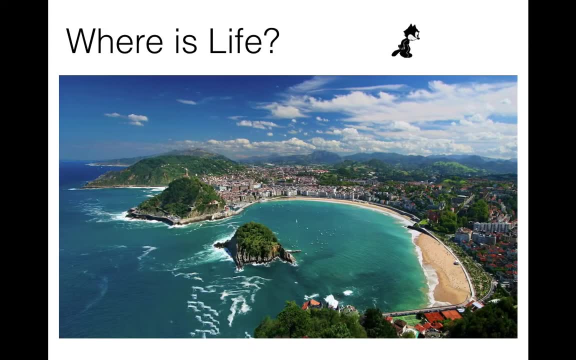 And it was 19th most cited paper in PRL back in these five years of span. Now We come to the part where we ask this question: Not what is life, but where is life? Okay, We asked it before: What is life? 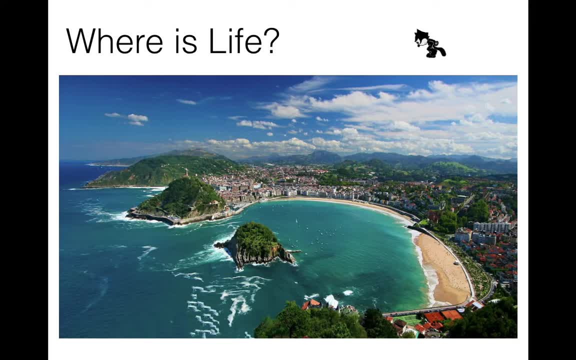 We know more or less what is life right. So back in the days when I was enjoying my time in this beautiful city doing postdoc- of course, Not surfing at all- It's a nice place. These places, natural places- are nice places to think about these fundamental questions. 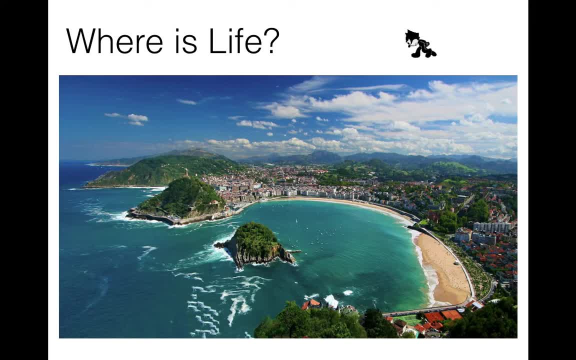 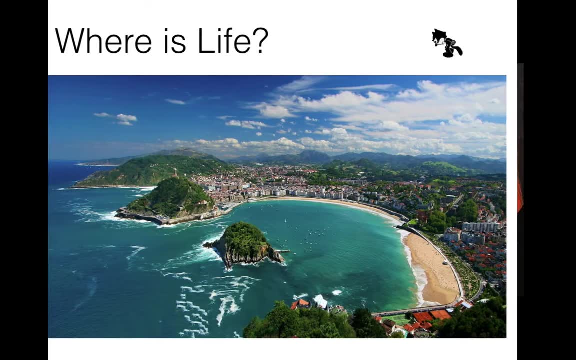 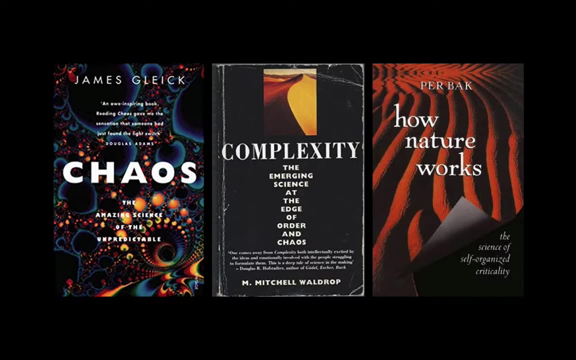 And I realized that everything that I had interest in somehow meet at one point Okay, And that point is the science of complexity. So basically, this course is about computational methods for material science, But that's a Trojan horse And to get the course in, then it opens and it's all complexity. 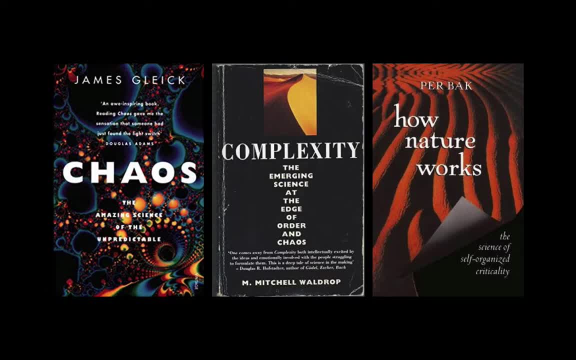 Do you understand the point? So I really recommend these three books to read, especially the middle one. Actually, no, not all of them. So how many books so far? Three books. Fourth is I'm a Strange Loop And Harvard Lecture. 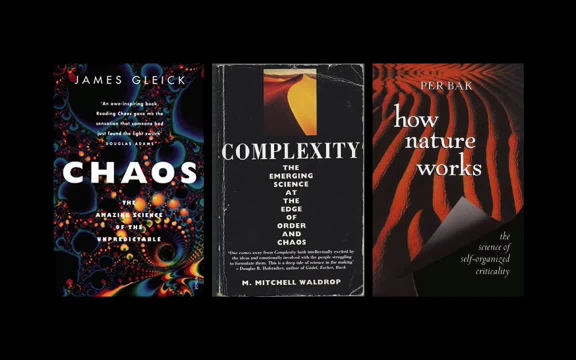 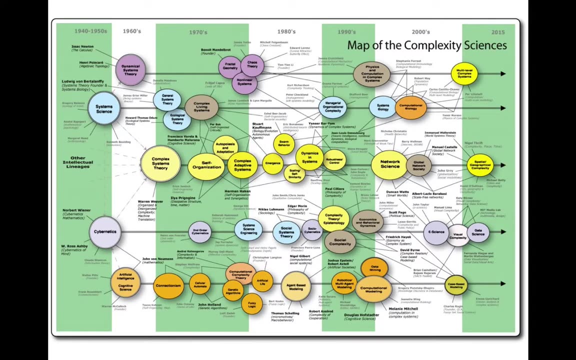 Don't forget. Okay, They will really click with this course if you read them. Okay, And you can see the emerging science at the edge of order and chaos, etc. And we will go through this map of complexity. So I realized that there is a science called complexity science or complex systems, whatever it's called. 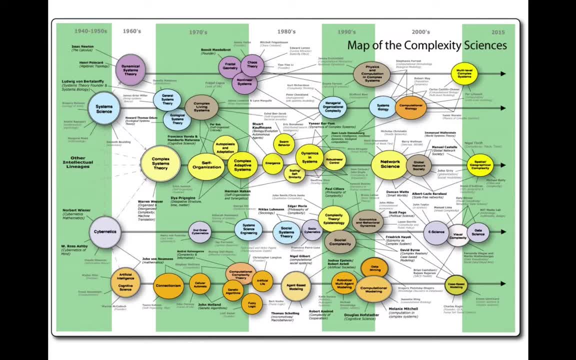 that brings together all my scientific heroes. So you can see it's a quite personal course, Okay, And we will go through many of these people. Like we already mentioned Von Neumann, We will mention Holland, We will mention Conway Wolfram. 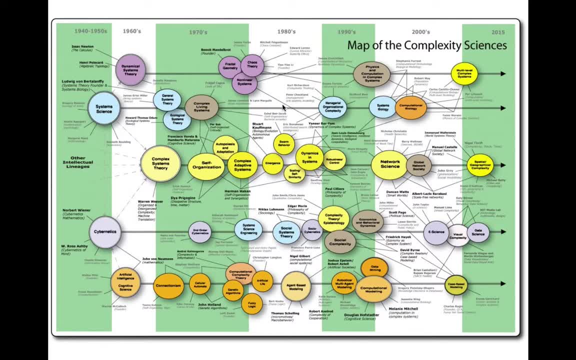 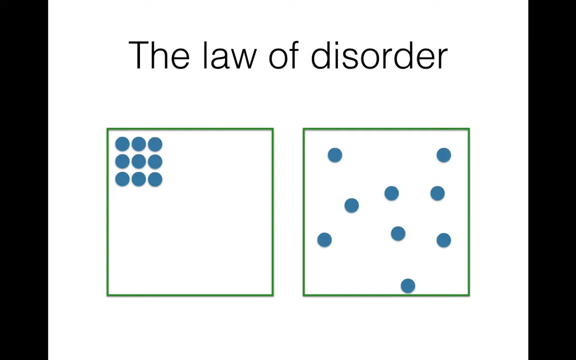 We will cover most of the dynamical systems. Mandelbrot, Mandelbrot, Everybody is here and they are together. Okay. So ultimately, if we think about everything in terms of computation, we realize that the ultimate force, like F equals ma, is a rule of physics right? 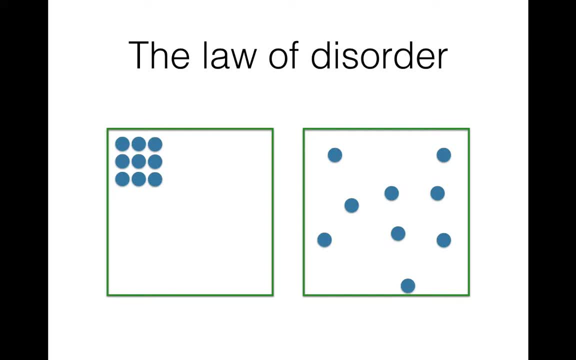 What is the deeper rule? Do you understand my point? Well, ultimately, yes, The deepest rules are still can be considered physical rules. But really, the second law of thermodynamics, for example, is more fundamental, to me at least, than if F equals ma. 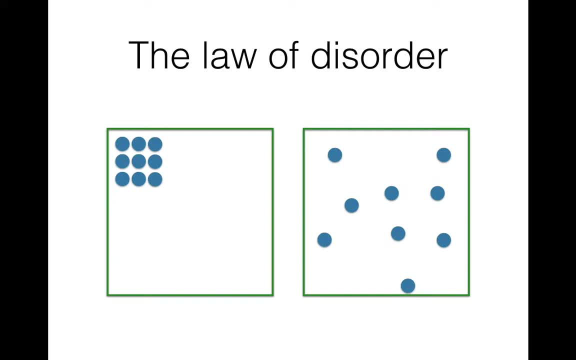 Okay, Because it's really really purely logical. If you take atoms in a corner, How many possibilities do you have? Like one, two, three, four. If you can arrange them anywhere else, you have infinite possibilities. So no matter what are the rules. 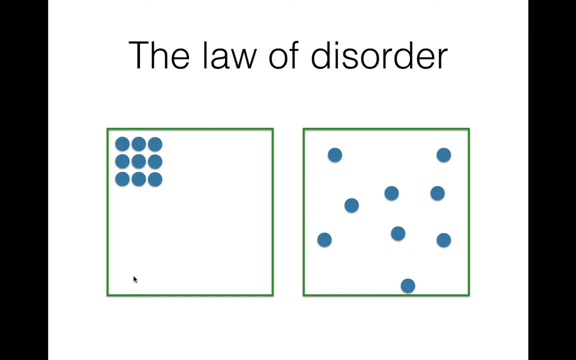 And we should, of course, take into account their interactions, the potential energy, whatever- But their dispersed version have more possibilities. Simply because of that, you will have a push towards disorder. So what I'm trying to say is that there is a probabilistic pressure towards disorder. 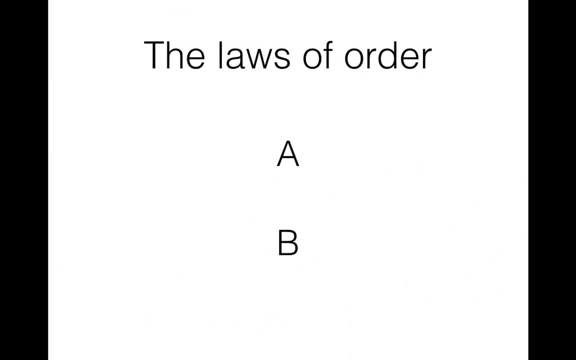 Okay, Let's skip this. But then why are we here? There has to be something that takes this disorder at the expense of creating even more disorder. Even faster, it produces some order. Did you get this point? And to have that, we need some laws of order. 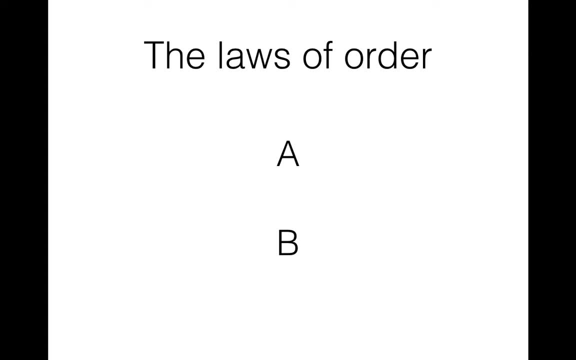 Fundamental laws of order, And here is one of them. You have A and B. These are chemicals. Okay, A and B comes together and creates can create AB, And another variant is creating BA. What if this chemical catalyzes that one and that chemical catalyzes this one? 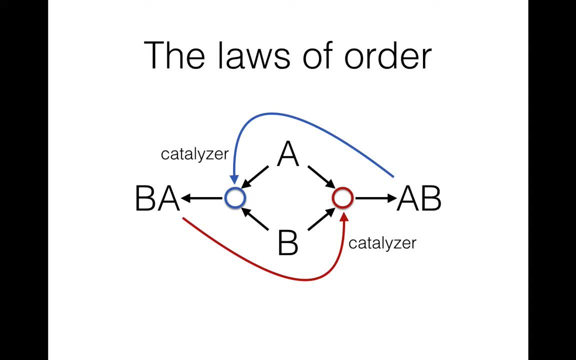 This is a straightforward feedback loop, But in real chemical metabolic networks, or in real chemical networks Or, how they say, autocatalytic reaction sets, There are chemicals that produce chemicals That produce chemicals That produce chemicals, Ultimately catalyzing the original reaction. 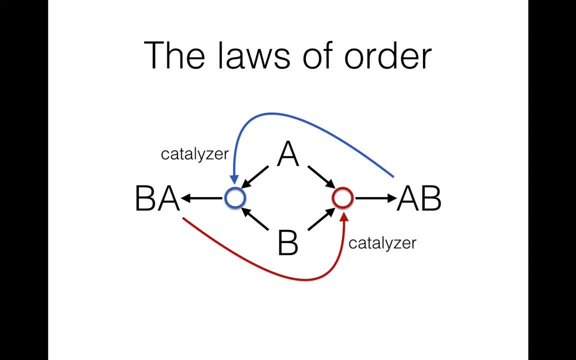 Do you understand this point? Hence, although things are going towards disorder, You will keep having these copies of these chemicals, And once you have those chemicals available, Then they will come together And if they create something that can reproduce itself, That's what. that's how life starts. 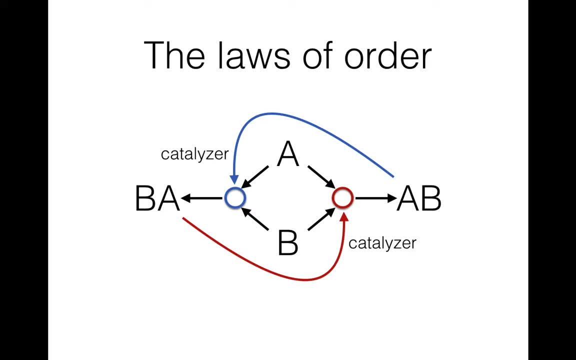 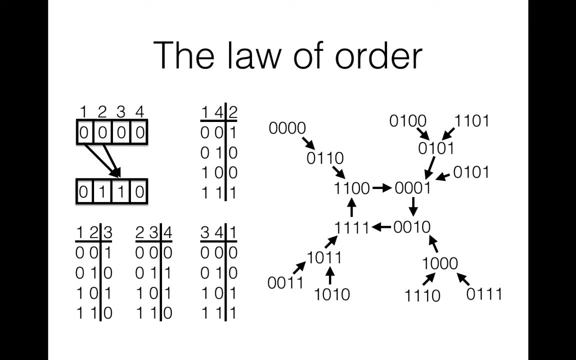 Right, This is another speculation, But one of my favorite origins of life theory, Autocatalytic reaction sets. Okay, And we are going to talk about Kauffman's ideas, Epigenetics And how he, by looking again at 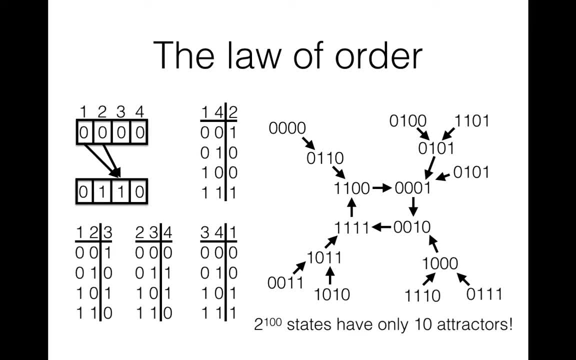 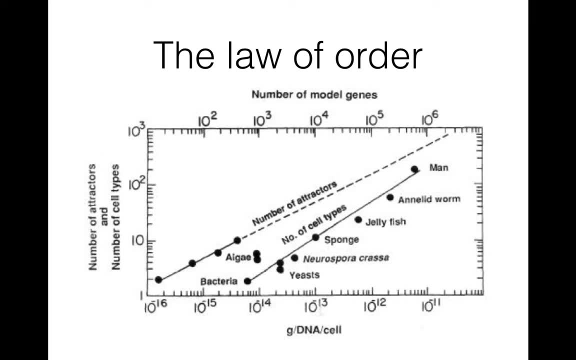 only at the computational universe He discovered that the types of the cells And the number of genes should have a logarithmic relation. Of course one can always criticize someone who is giving a log-log plot And saying that it's linear. Believe me, everything in log-log plot looks linear. 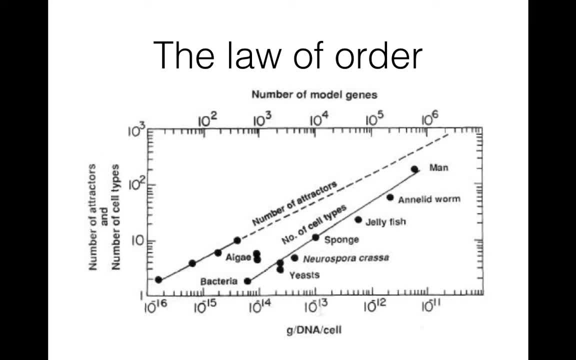 Okay, But still it's something, And at during the course we will discuss it in a detail And we will understand what's going on here. You can see that from bacteria to man, They are in the same linear Well. jellyfish is out. 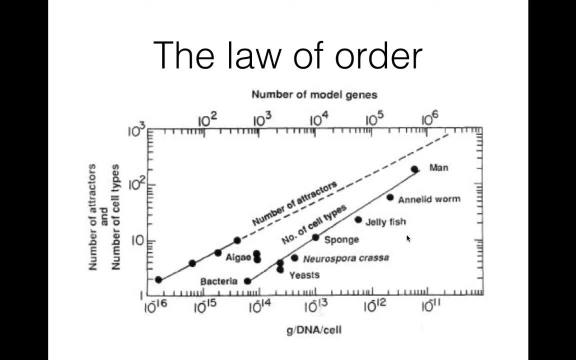 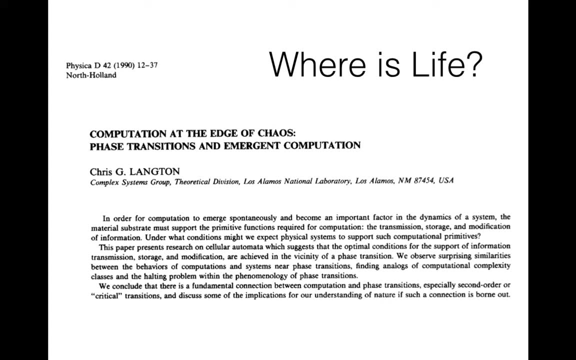 But sponge man and bacteria. That's impressive, Right, Okay, So again, where is life? So the ultimate, the last speculation of today's lecture is that life arises when chaos and order meet, When disorder and order meet, When you have these two powerful laws against each other clashing. 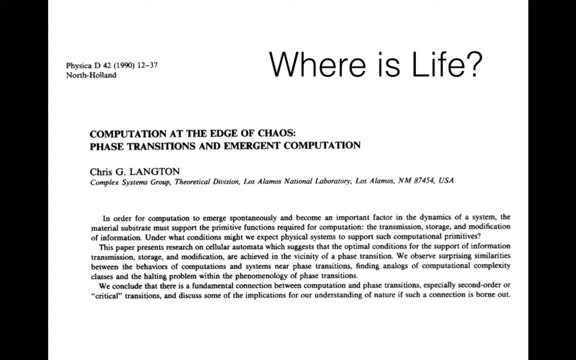 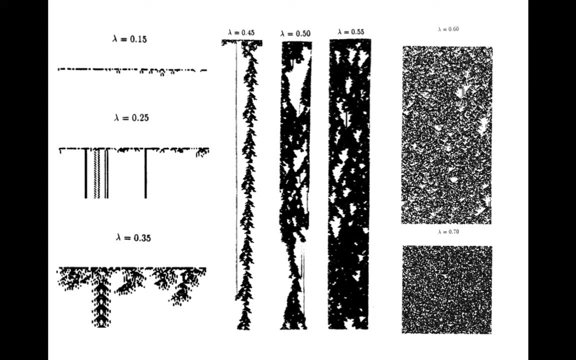 And they create these beautiful structures. And someone tried, to many people tried to formulize it, And one of them is Chris Langton, Who looked not only just rule 30.. But all possible one dimensional automata's Whereby you include also the second order interaction. third order, nth order. 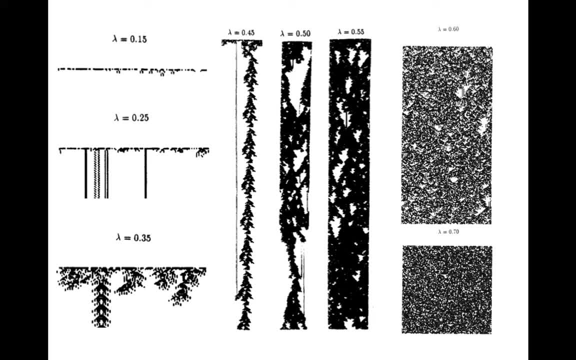 Doesn't matter. And there is this lambda parameter that is used, And when you start from lambda, very small, You get killed by a bus. Okay, You see No life, Then this is where you are alive. But as one of the songs of Radiohead says, 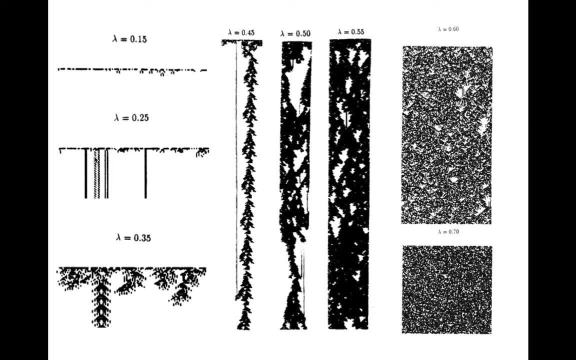 A job that kills you. You know No surprises. This is more interesting job, Okay, But you are still going to job. To work home, work home. You are happy, Very exciting, But repeats What was lambda. 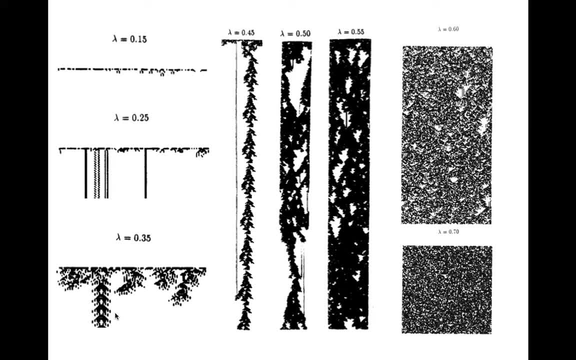 What is lambda Here? lambda is, By the way, I have a better lambda, Believe me or not. I am writing a paper on it, Hopefully, No, no, no, This lambda is okay, But I have a better lambda. 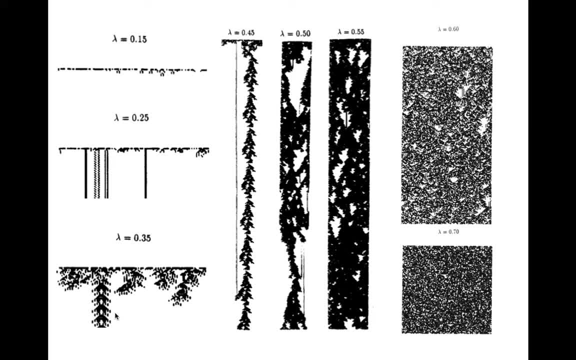 Which was inspired by giving this course previously. So This lambda tells you the probability of having one in the next run. So if you take into account all possibilities of the upper layer, What is the probability of this one being one? Okay, So he claims that when lambda is 0.5. 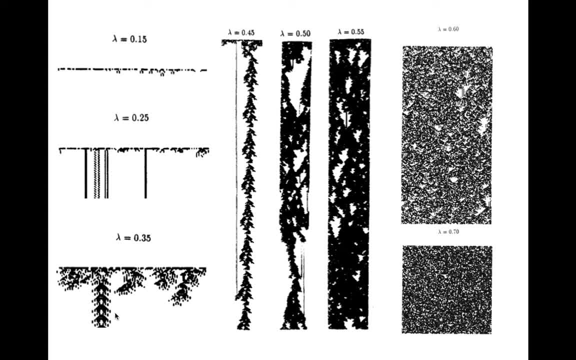 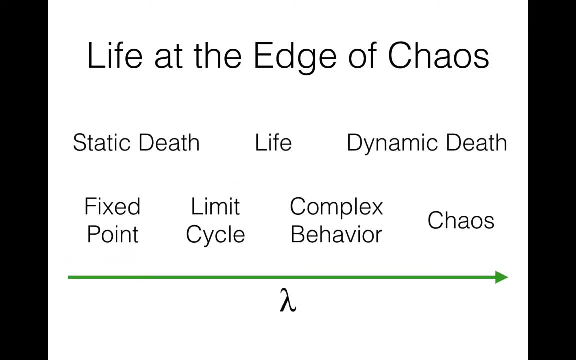 When it is near to it. At that point Then you would reach The maximum transient. You can see that it never repeats. Very interesting. So let me make my point. You have fixed point, limit cycle, complex behavior or chaos. So basically you have static death or dynamic death. 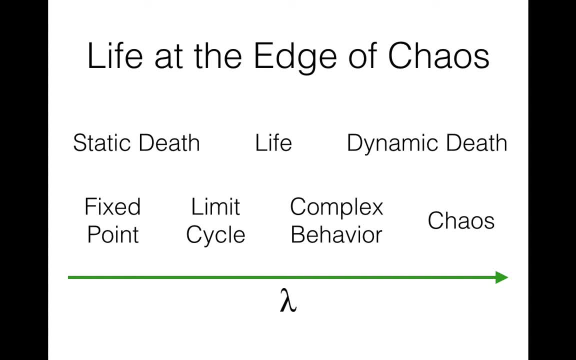 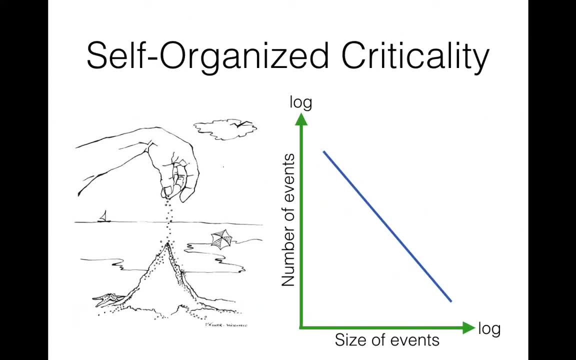 And when these two deaths meet, You have life out of it. Okay, And There is actually. Most of the systems Are self-organized to this critical point Where You have maximum Entropy, Maximum information processing. Actually, maximum entropy is 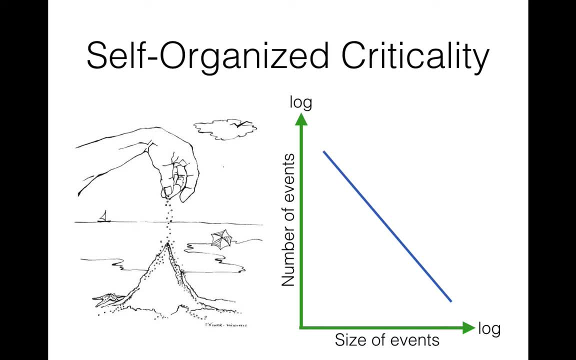 Bad, It's the chaotic death, But Anyways, Maximum aliveness Production, Wow, Okay, We should speak about it a lot, Maybe. Yes, Very good, Anyway, And This is the book That: How nature works. 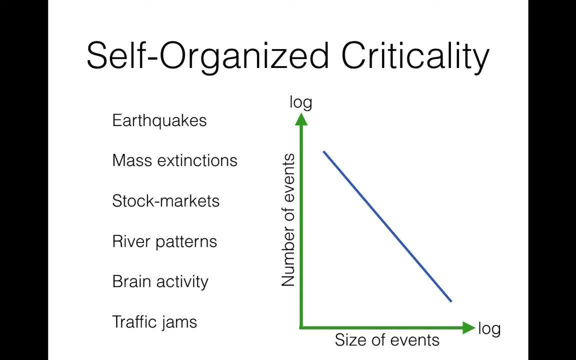 Do you remember that book? That's where The person Explains How He accounts for earthquakes, Mass extinction, Stock markets, Etc. And We are going to Deal with this one as well. So, Okay, How nature works. 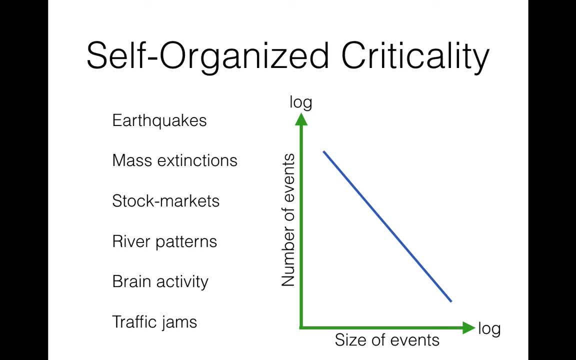 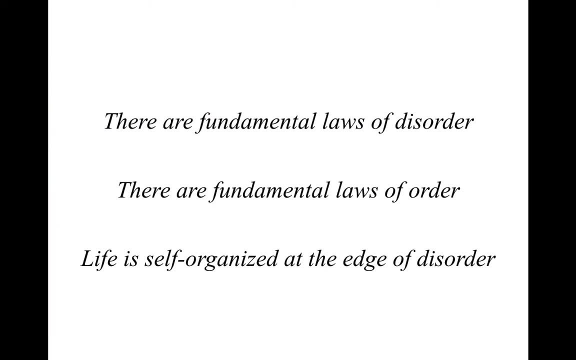 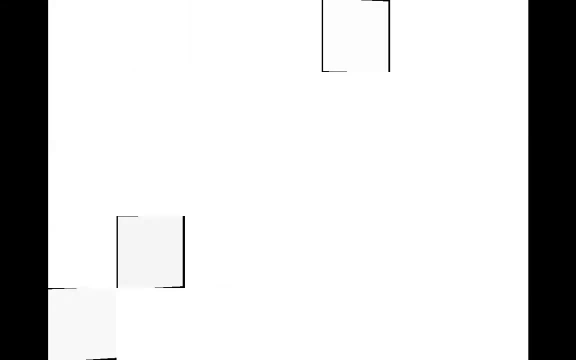 Disorder. Okay, Now Let's make a philosophy out of this. Remember: All here is good. Nothing is evil here, Okay. So Good order, good disorder, one of them. there are always these two choices: safer choice, more possibilities like knowledge, imagination. okay, what I'm trying to convey here is that the way to reach this maximum efficiency of being alive is being in between. 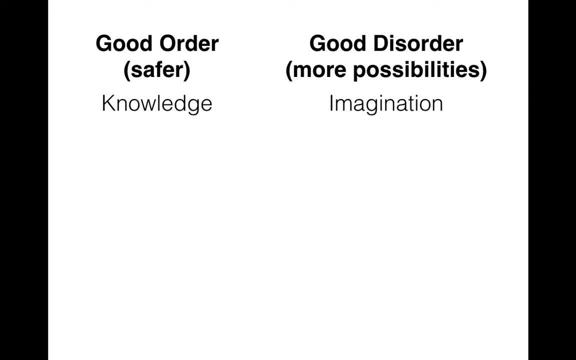 like having more, as much knowledge as possible, but while having, while not restricting imagination, like if you read all the books, it might restrict your imagination. you might not write a new book. do you understand my point? and what is Einstein's word? his imagination is more important than knowledge. 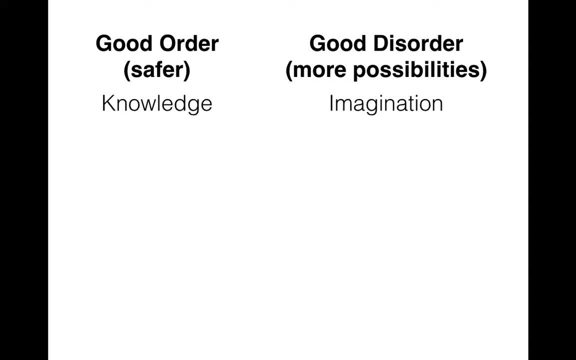 that's something that's okay. this is my. my ultimate speculation is that the right one is slightly- I mean- more safer, although this says it's safer. if you want to keep yourself alive in maximum entropy production state, then you should take into account this one. saving- investing doesn't make sense. saving safe- it's underneath your pillow. 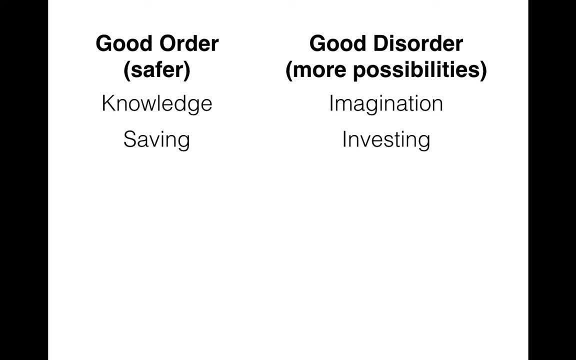 or investing, making it more at a risk of losing, of course, security, trust. we are going to look at this algorithm, tit for tat algorithm that would, if you play together, okay, do we have like 10 more minutes? yes, it's 5.30,. right, let me make it more clear because my time will run out. 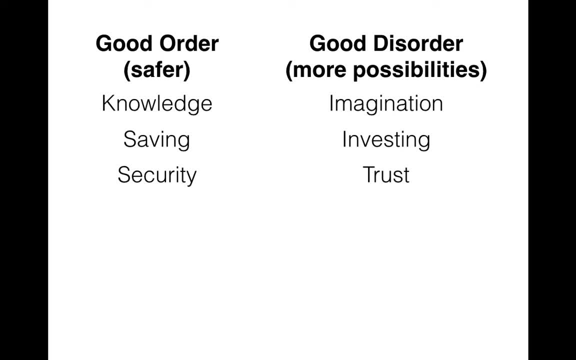 in two minutes. do we have 10 more minutes? so there was- and we are going to look at this paper, where they make a tournament of algorithms and the game is called, like evolutionary game theory. that's the subject. so we play with each other. I give five, you give five, we both take five. 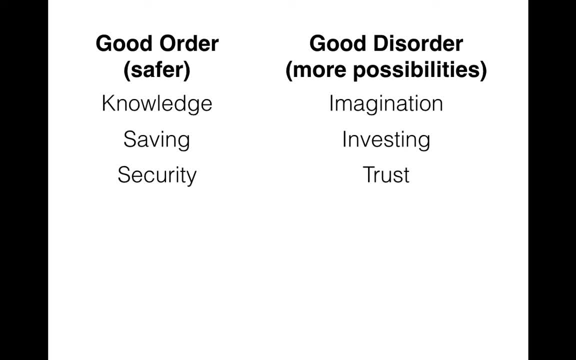 I give five, you give five, we both take five. you give five, you give seven, we both take six. so in a way I defected you. you were cooperative, I was uncooperative. I won, but only for a moment, because you know that I am a five giver. do you understand, the next time you are going to give me one, depending on the algorithm that you have? and the algorithm that is unbeatable so far is tit for tat. 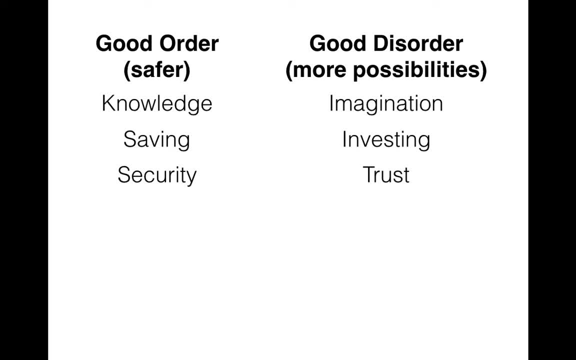 it gives you whatever you gave the last time, do you understand? but what it should give at the first time, it gives 10, the maximum of positiveness. so that kind of supports my point of being slightly on the side with more possibilities. do you understand my point? 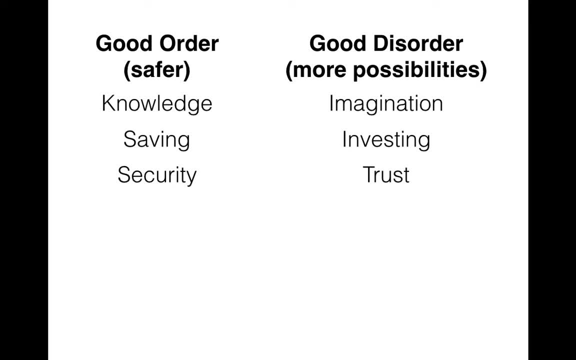 and being on the side of trusting people rather than securing yourself from them. unity, diversity makes sense. linear non-linear makes sense. we can speak an hour about it- conservative, liberal- getting into too much politics- but it's really not a political issue. 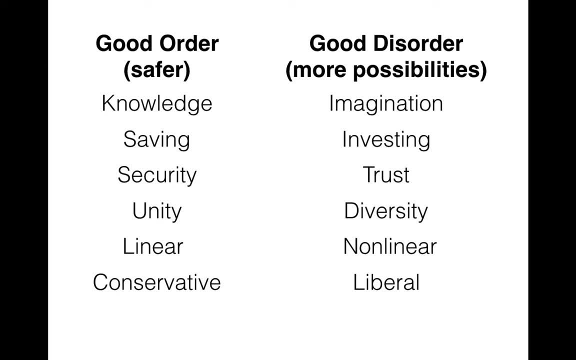 notice that usually we are these liberals in the universities, right, notice that I'm talking about the importance of being conservative as well. do you understand my point? if you are ultra-liberal, you lose your identity at some point. you become this entity in computational universe, but